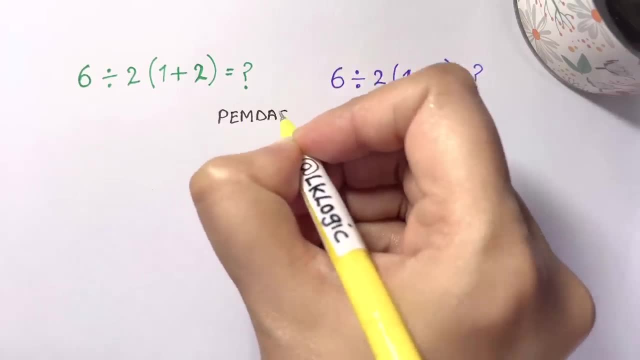 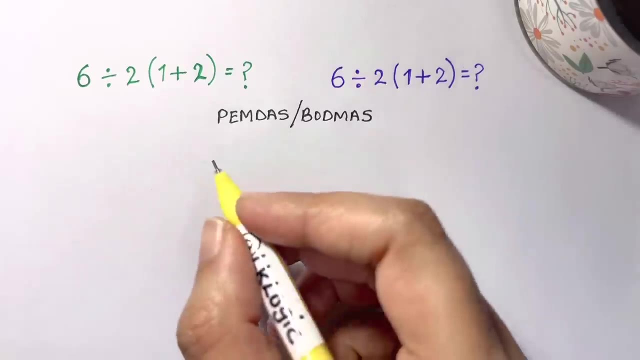 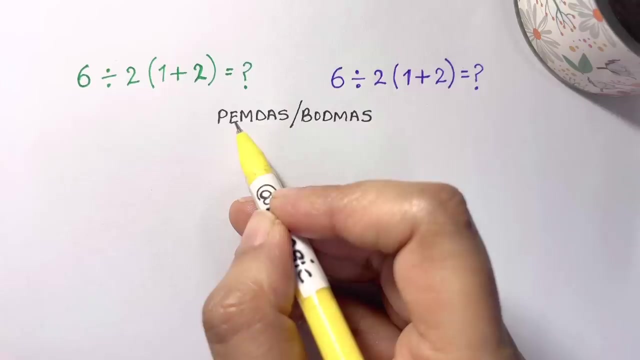 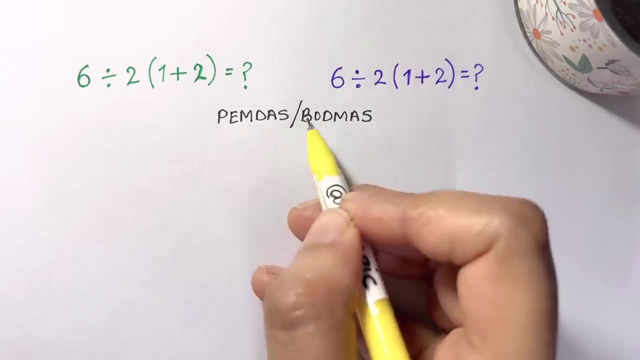 PEMDAS or BODMAS. This refers to evaluate parentheses or brackets first, then exponents or orders, then multiplications and divisions and finally additions and subtractions. So parentheses and brackets are same exponents or orders, multiplications, divisions. 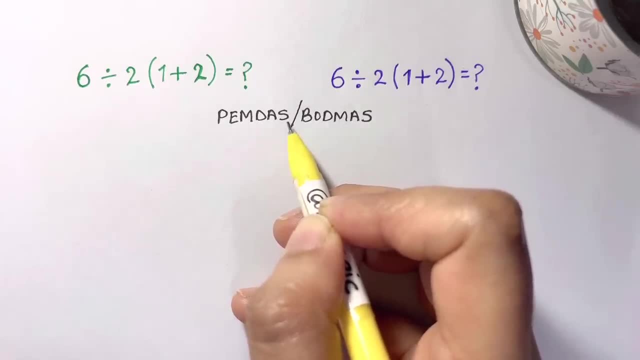 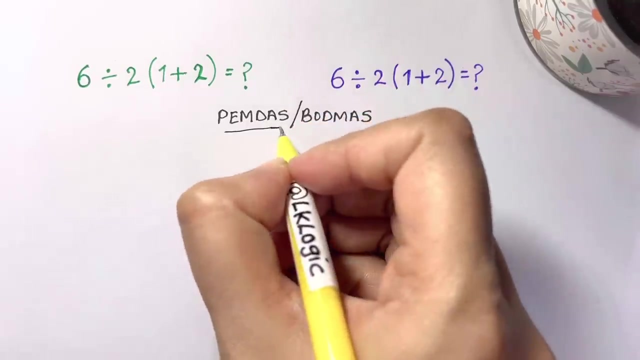 and then additions and subtractions. If there are two operations of the same precedence, like multiplication, division or addition subtractions, then you have to evaluate them from left to right, From left to right. The first step of the problem has no controversy. 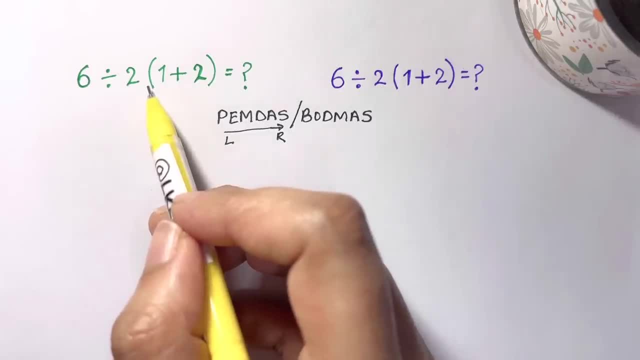 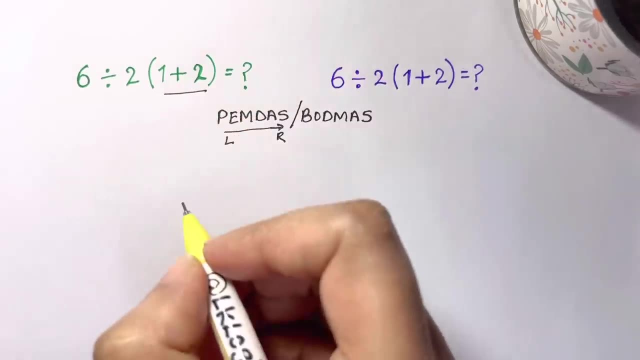 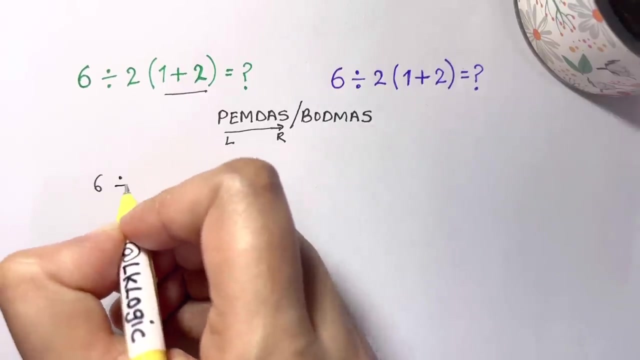 So we can just solve that This expression contains a parenthetical expression which must be evaluated first. One plus two is inside the parenthesis, So we will evaluate one plus two to get three. We have six divided by two parenthesis. One plus two is three. Now the 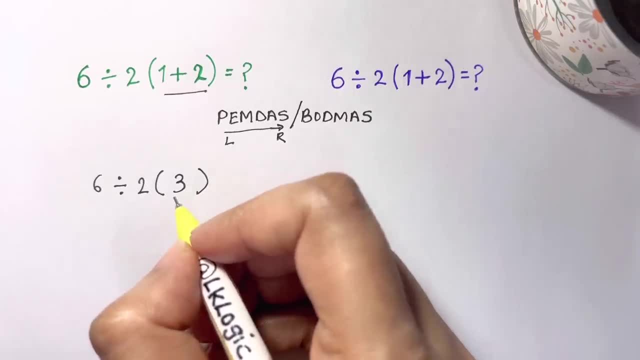 question is what to do next. If you input this into Google or any other side of a calculator, the thing that's going to happen next is all of these will interpret the parenthesis as an implicit multiplication. So this two parenthesis three will be converted to two times three. 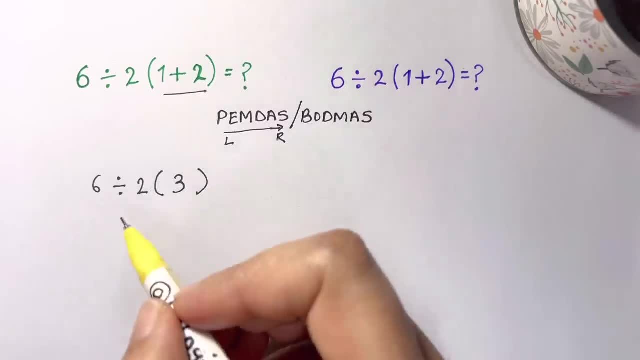 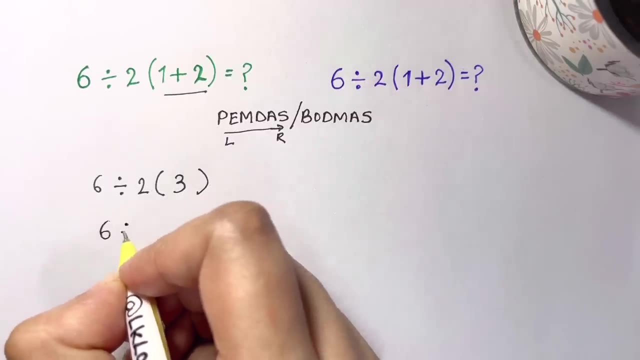 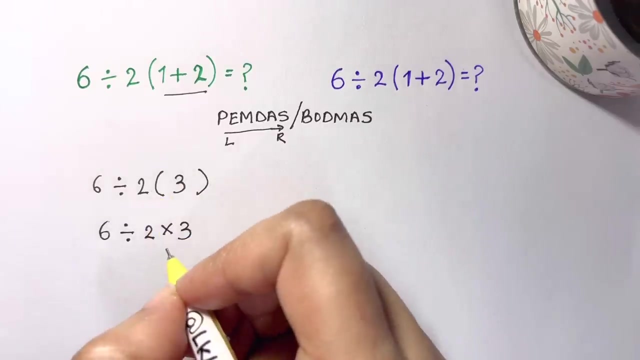 Now we're going to continue with the order of operations. This expression only contains multiplication and division. So it's like six divided by two times three. The parenthesis is converted into multiplication. This is a multiplication and division equation. So this is going to form one minus 3 divided by 3.. So this is going to become one minus 3,. 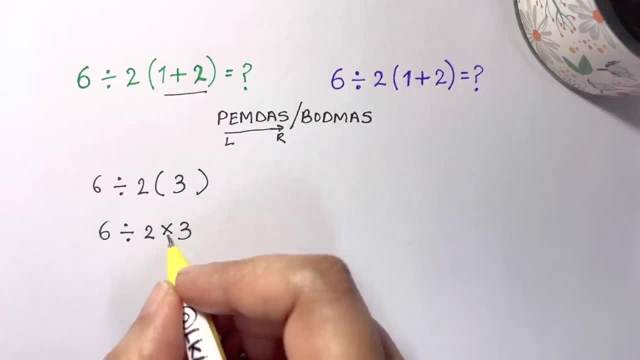 These are operators of equal precedence, division and multiplication. So we evaluate from left to right. So when we evaluate from left to right, we have this 6 divided by 2.. So, starting on the left, we have 6 divided by 2, which is equal to 3.. 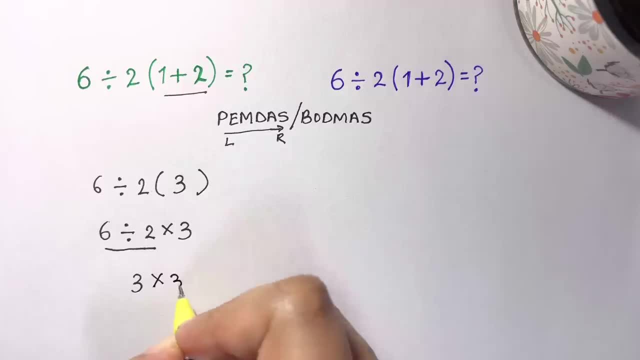 And then we have 3 times 3, which is equal to 9.. So the one final multiplication is equal to 9.. That gets us to the correct answer of 9.. That's according to the modern usage of order of operations. 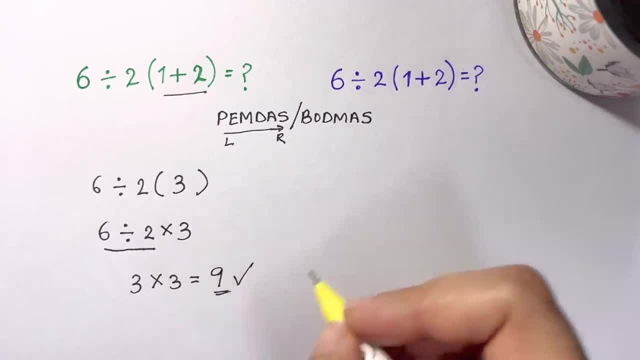 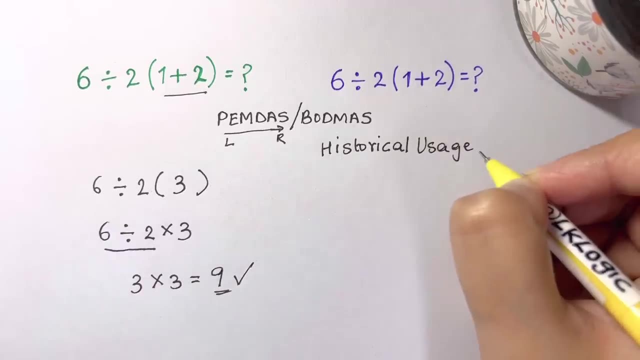 So why did the problem cause so much controversy? Well, there's another answer: from historical perspective. So I actually found some documentation that the order of operations did have slightly different understandings In certain texts in 1917 or before. So the first part is same as before. 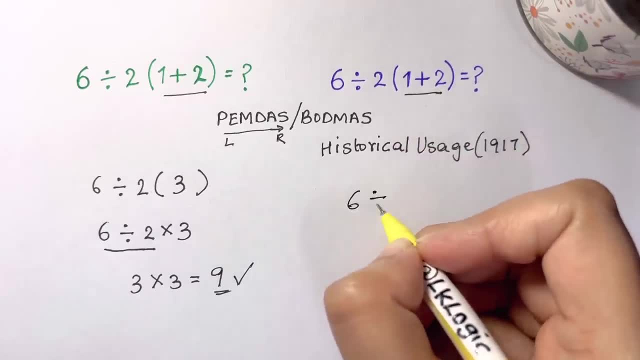 1 plus 2 can be written as 3.. 6 divided by 2 times 1 plus 2 is 3.. The debate that comes around is the division symbol. So what is 6 divided by 2- parenthesis, 3 equals 2?. 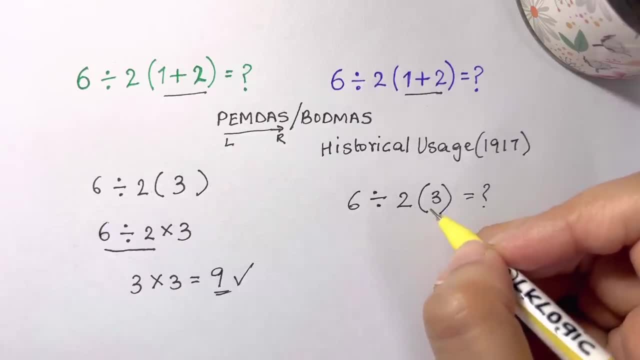 Well, there were textbooks a lot of use. They used to say that if you had something on the left divided by something on the right, Left divided by something on the right, This was understood to mean that you want to divide the entire product on the left with the entire product on the right. 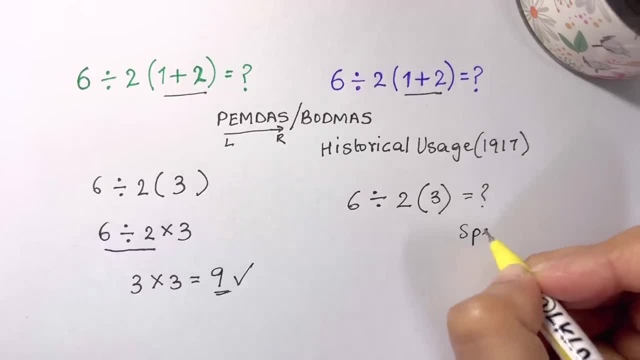 That's a special rule. What's that special rule? Well, the entire product on the left is divided by the entire product on the right. So, for example, if a textbook wrote something like this: X divided by 2Y, So that's equal to X over the product of the denominator. 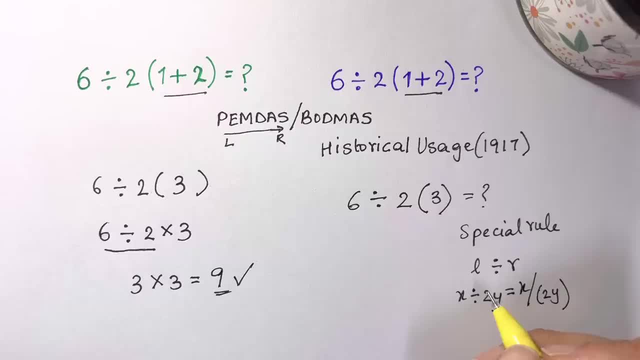 That's parenthesis 2Y. So under this special usage, which is an exception to the order of operations and we don't use it anymore, So applying this rule, what happens is. So applying this rule, what happens is. 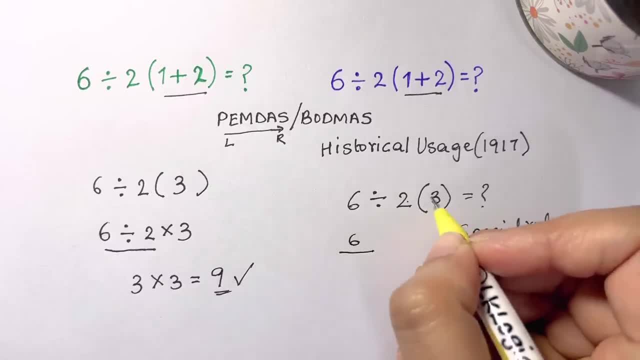 You have: 6 divided by 2 multiplied by 3 is the product of complete denominator Now, which is equal to 6 divided by 2 times 3, is equal to 6 divided by 6, which is equal to 1..